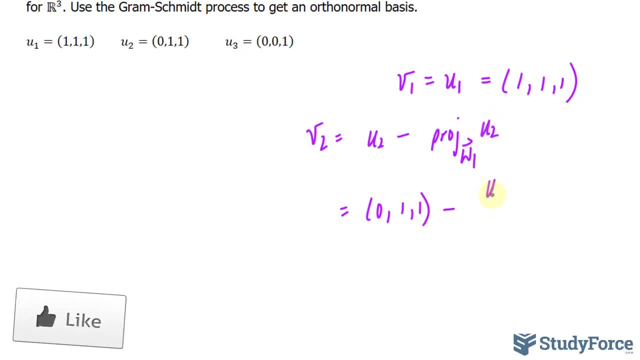 we take the inner product of U2 and V1 over the norm of V1, raised to the power of 2.. And all of this is being multiplied to the vector V1.. So let's start off with the numerator. We need the inner product of U2,. 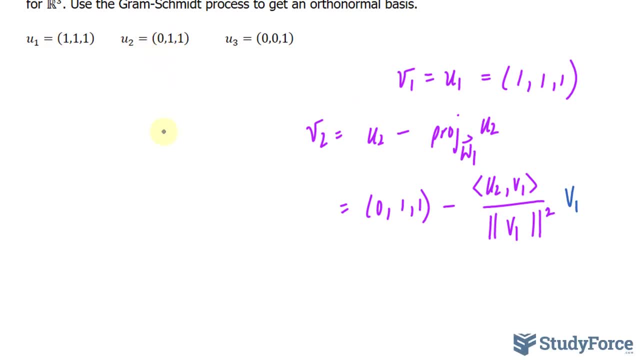 and V1.. For that we multiply each component, then sum that up. So 0 times 1 is 0.. 1 times 1 is 1.. 1 times 1 is 1.. This part becomes 2.. To find the norm of V1, notice that it's being raised to the 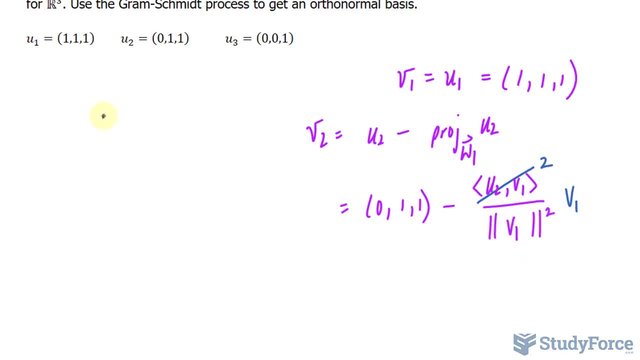 power of 2.. That's important, because to find the norm of a vector you do the following: You find the inner product and then you raise it to the power of half, But since this is being raised to the power of 2, the 2 and the half become 1.. And then you raise it to the power of 1.. And then you 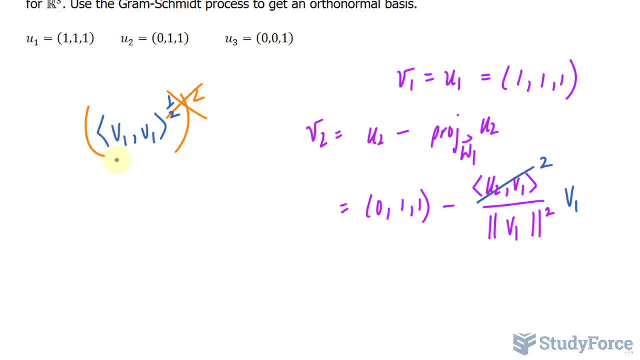 raise it to the power of 1.. So we don't have to worry about that part. All we have to find is the inner product of V1.. Remember V1 had these components. So 1 times 1 is 1, plus 1 again. 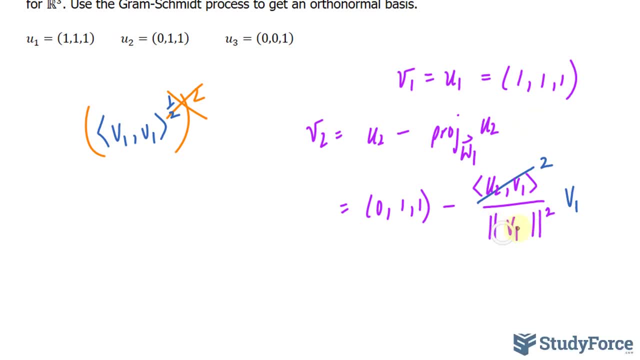 plus 1. That gives us 3.. So the bottom part here is 3.. We have 2 over 3 times the vector V1. Let me just replace that with its components. So we end up with to find V2, we have to subtract. 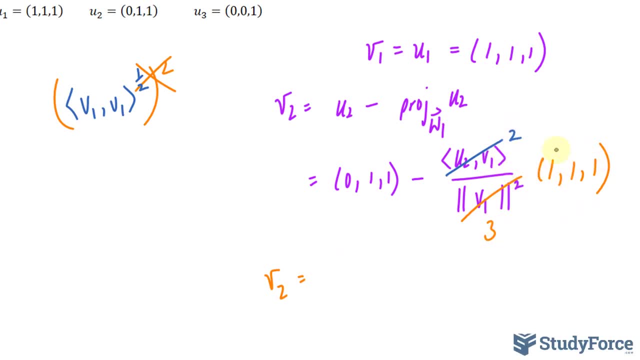 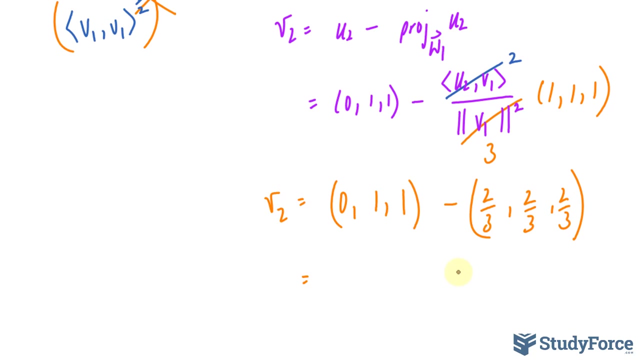 this vector with 2 over 3.. 3 times this vector, I have 0, 1, and 1, minus 2 over 3, 2 over 3,, 2 over 3.. 0 minus 2 over 3 is 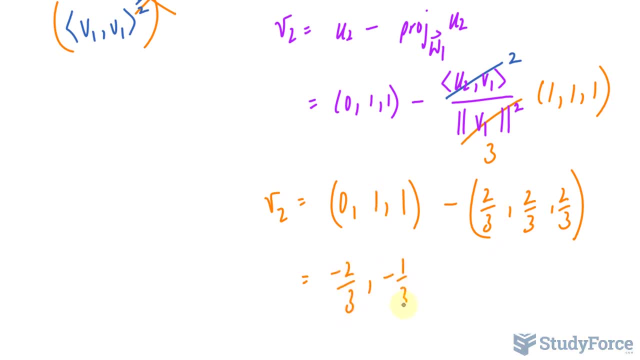 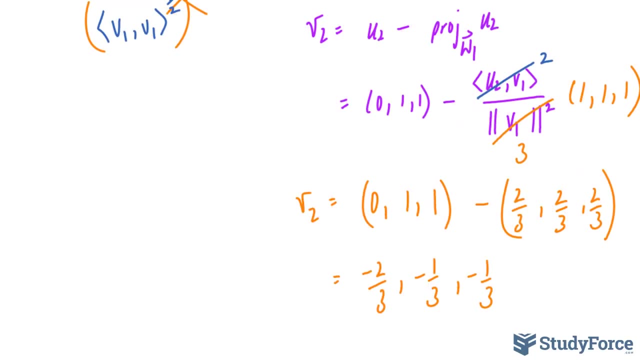 negative: 2 over 3.. 1 minus 2 over 3 is negative, 1 over 3.. And 1 minus 2 over 3, again is negative: 1 over 3.. That right, there is V sub 2.. Okay, now we have to find V sub 3.. And to find V sub 3,. 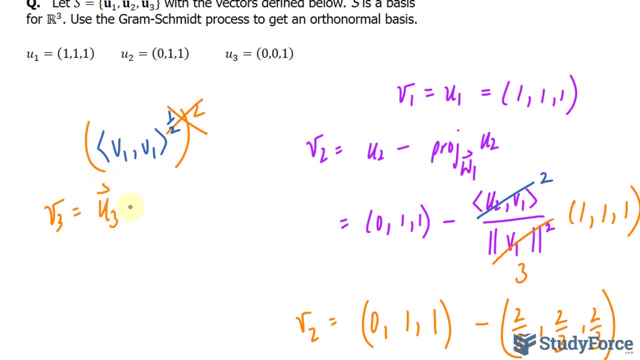 we will be subtracting U sub 3 with the projection of U sub 3 onto W sub 2.. And just to be clear, that right there represents the space span by V sub 1 and V sub 2.. So space spanned. 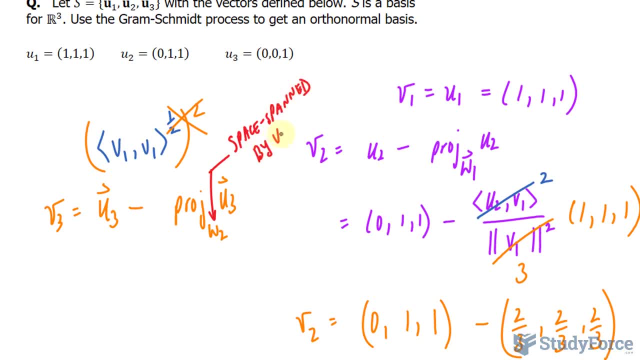 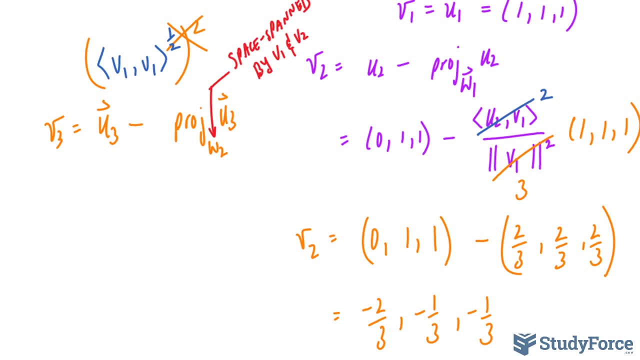 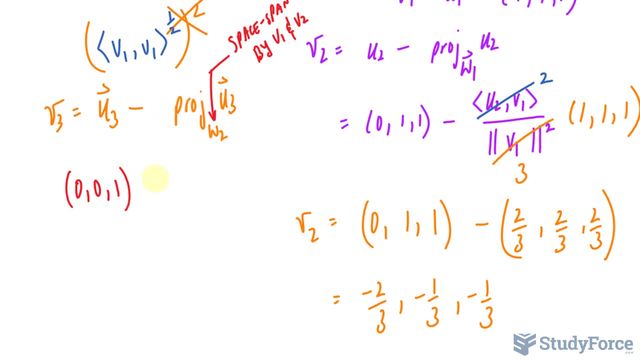 by V1 and V2.. So how do we represent the space span by V1 and V2?? Well, this part we already know is a vector and it has the components 0,, 0, and 1.. This part is: 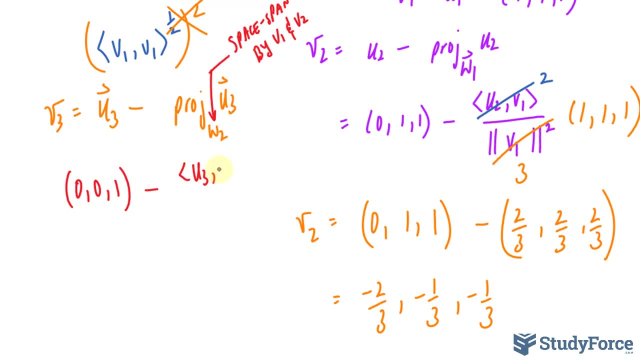 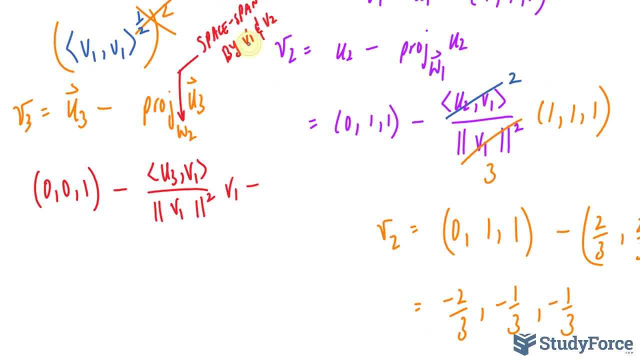 represented as U sub 3 and V sub 1, over the norm of V sub 1, raised to the power of 2.. And that's being multiplied to the vector V sub 1.. Minus, remember it's spanned by V sub 1 and V sub 2,. 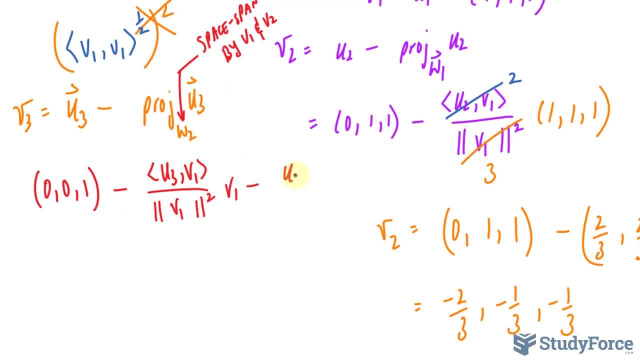 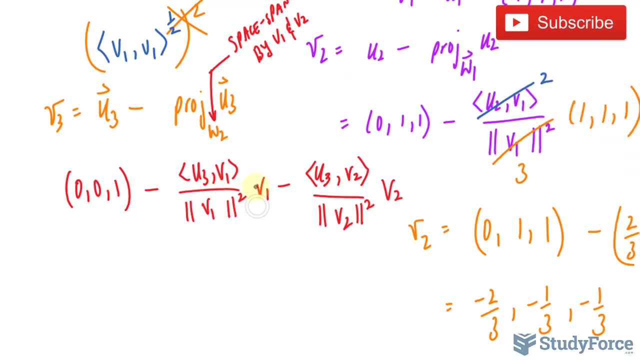 so we'll repeat that, But with V2.. So, as you can tell, there's a lot of work involved here And we'll repeat the steps that we did previously over here and over here, And it's going to take a while to do So. just to: 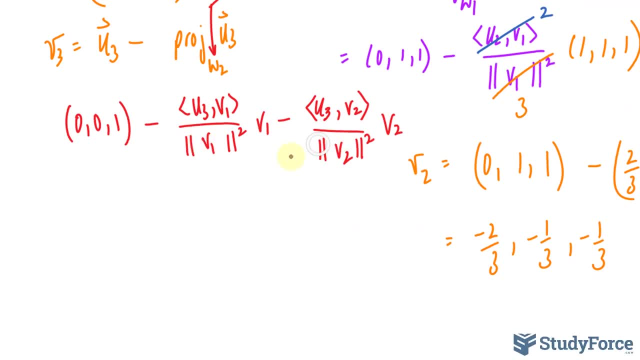 save some space, I'll just write out what you should end up with for these two expressions, So that one stays the same And remember we're finding vector V, sub 3.. We have 0,, 0, and 1.. 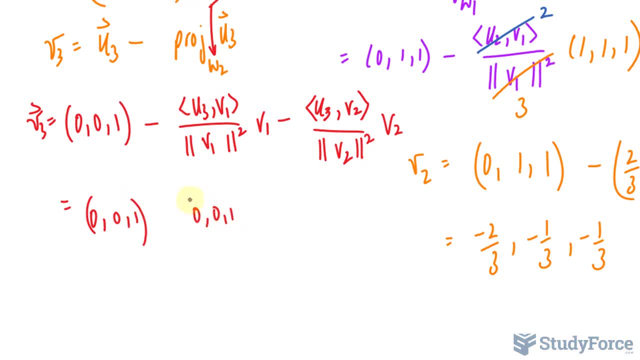 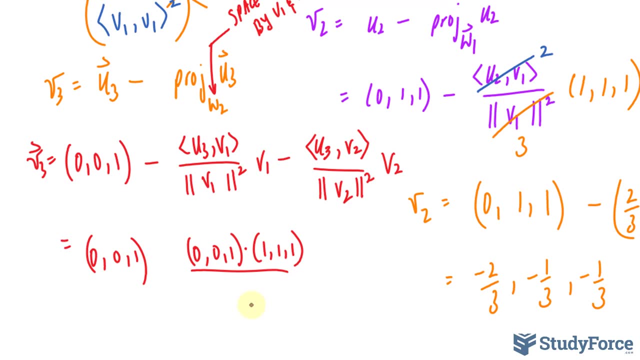 Over here we'll have 0,, 0, and 1.. Multiply 2,, V sub 1,, which was 1,, 1, and 1, over the bottom should become 3.. It's the same thing as. 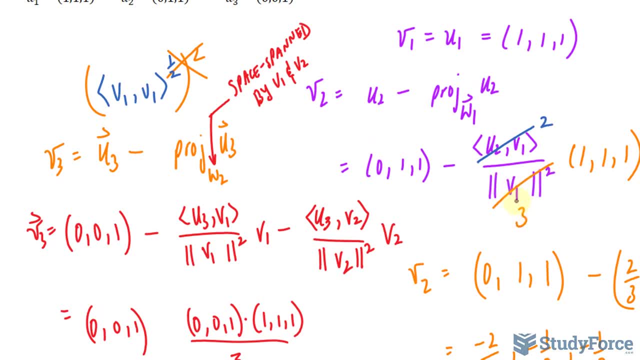 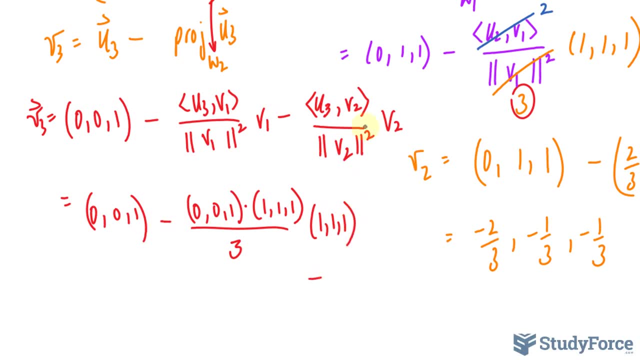 before remember Where we had this part and we wrote down 3, times the vector which has these components minus. now this part is going to be new V2, we found was this, So we'll be using this: 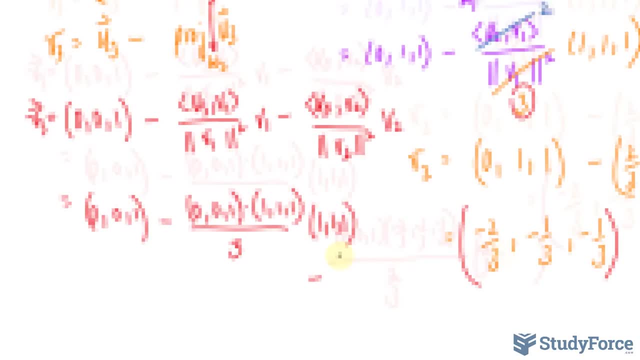 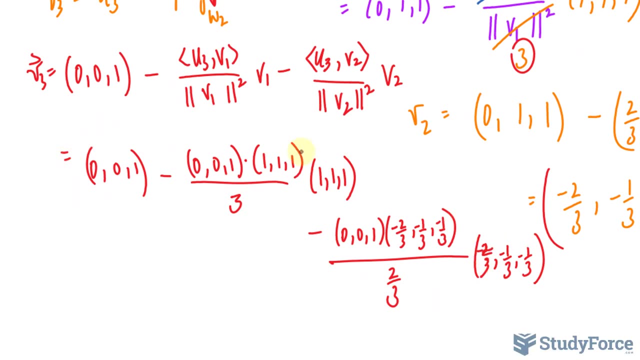 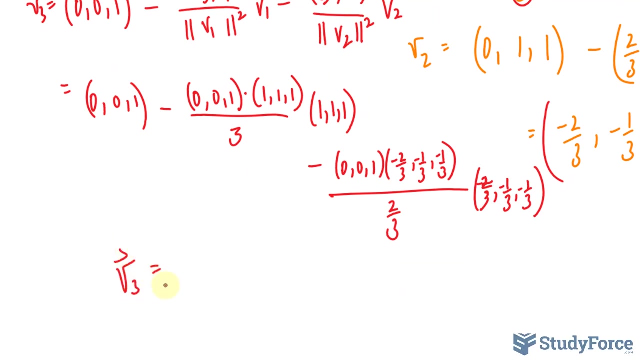 information, along with U sub 3,, and you should end up with the following: Okay, so now you have to subtract all of these together And that will end up giving you V sub 3.. If you do that correctly, your vector should be 0,. negative half and positive half. 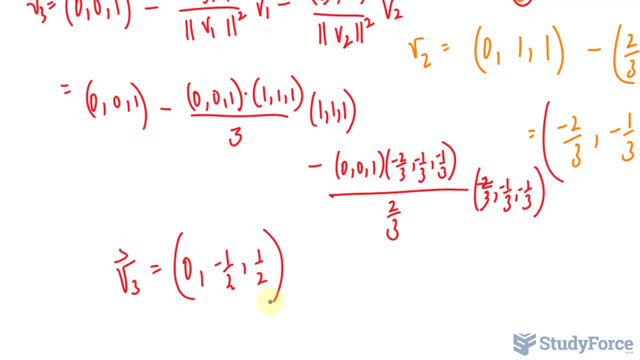 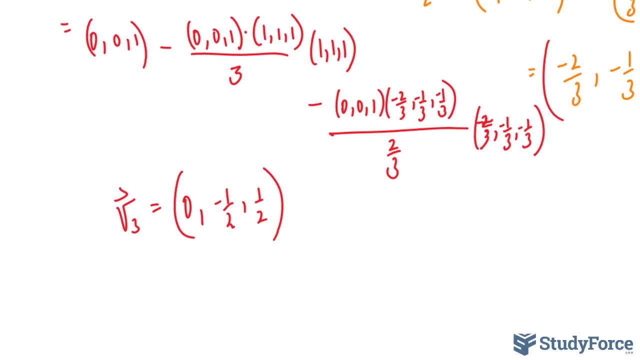 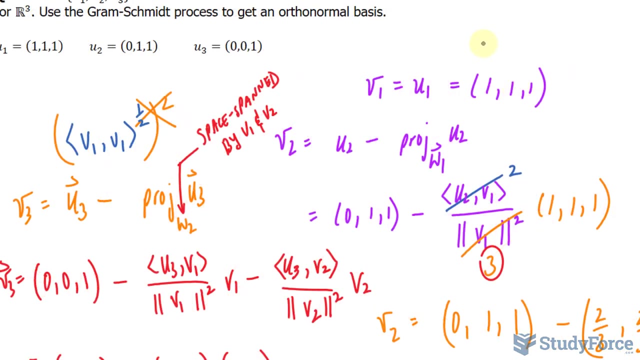 To get the orthonormal basis, we divide each vector- V sub 1 through V sub 3, by its norm. So now we have to find the norm of each of these. Let me go back to this one. To find the norm of V sub 1, we will take each of these, multiply it in. 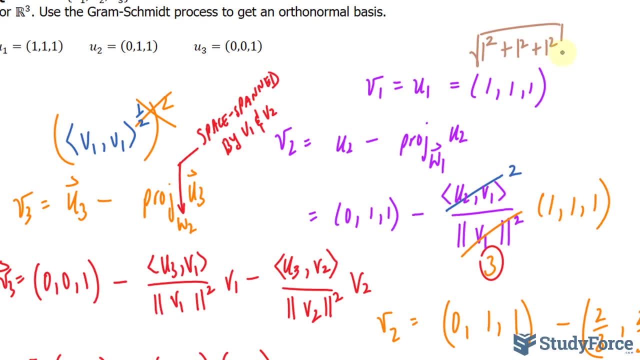 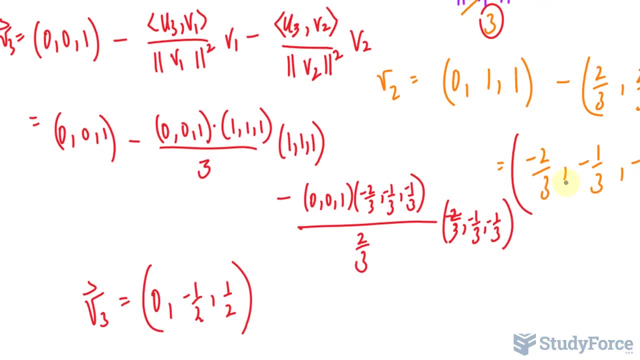 itself and square root it. So we get the square root of 3 for here, For V, sub 2, remember that was our answer And the norm of this one. if we square each of these and subsequently square root, we get. 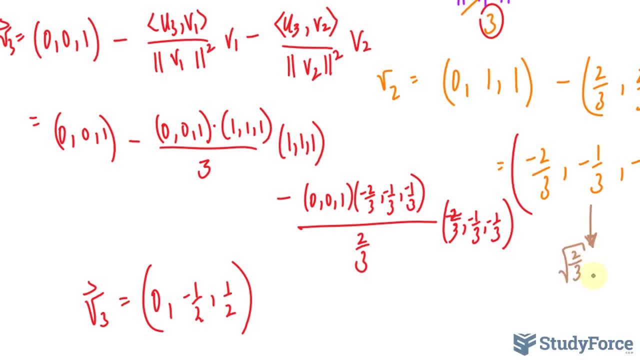 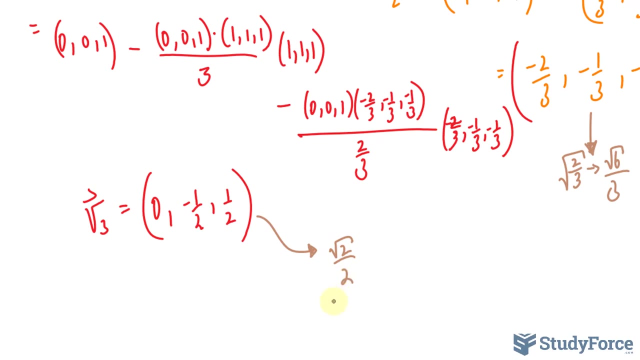 the square root of 2 over 3.. Which happens to reduce down to the square root of 6 over 3 once we rationalize- I'm not going to show that step- And if we find the norm of this vector, we end up with the square root of 2 over 2 after we rationalize. 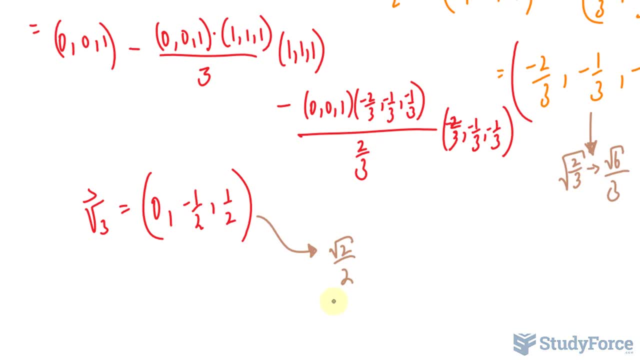 As you can tell, I'm not showing you how to find the norm. It's assumed that you know how to. We do have videos dedicated to that, if you still need more assistance. So I'll divide this by that expression, this vector, by that expression and 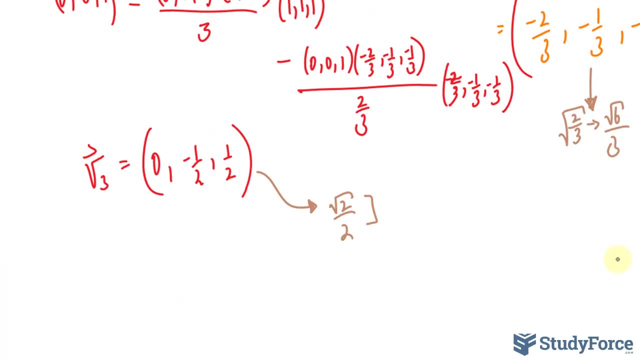 vector by the square root of 3.. And we end up with three new vectors, which consists of our orthonormal basis. So our orthonormal basis will be 1 over the square root of 3,, 1 over the square root of 3, 1 over the square root of 3.. That is. 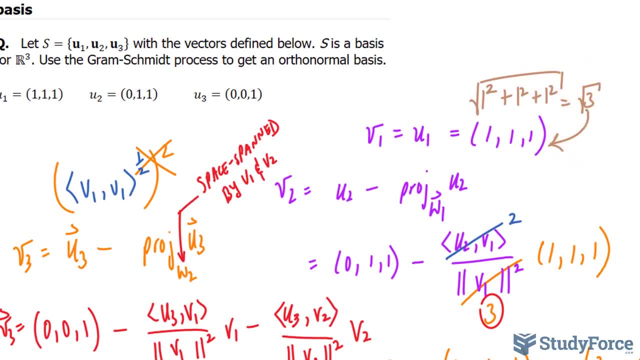 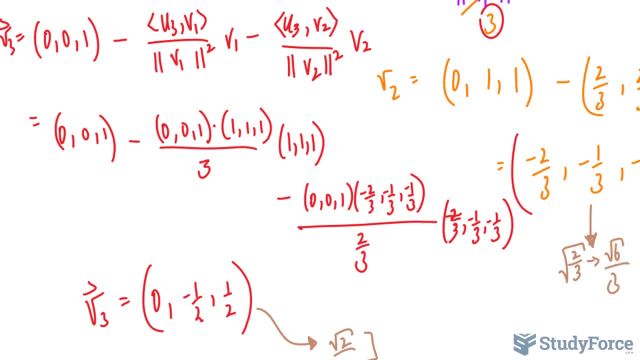 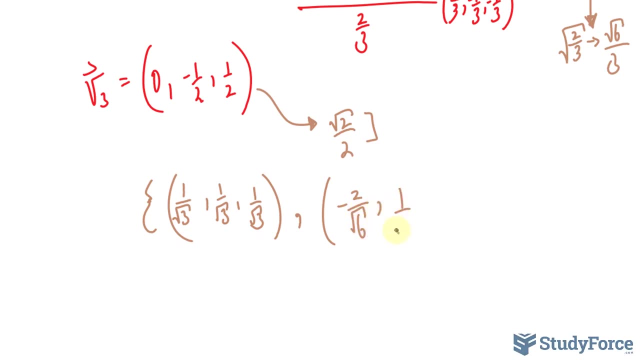 associated with this part. And then, when we divide each of these by the square root of 6 over 3,, we'll end up with negative 2 over the square root of 6, 1 over the square root of 6, and 1 over the square root of 6.. And doing the same, 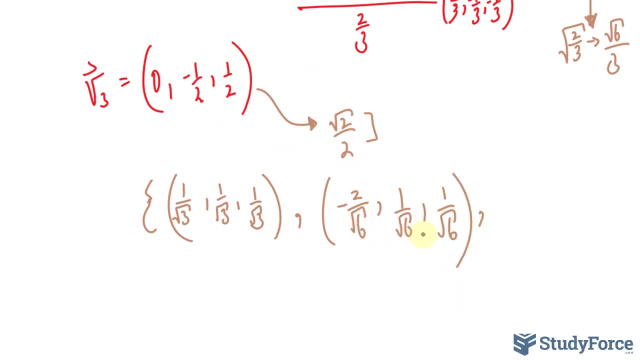 thing here. And, by the way, if you don't like the fact that we have square roots at the bottom, you can rationalize each of these components. It's the same thing. And lastly, for over here, we get 0, negative 1 over the square root of 2, and. 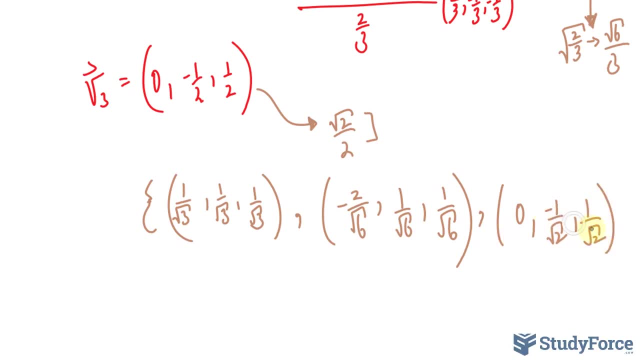 1 over the square root of 2.. Once again, you can rationalize these last two components. So this right here represents the orthonormal basis using the Gram-Schmidt process. And there you have it. That is how to use the.